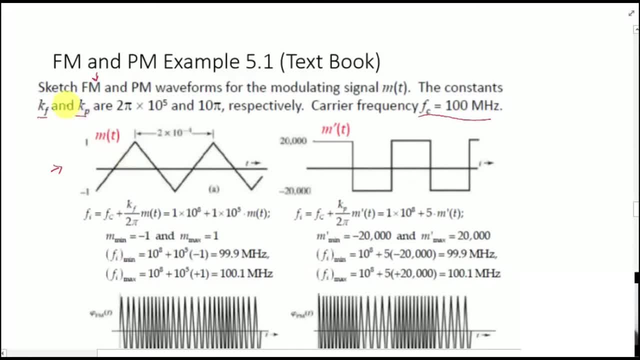 based on this and on these parameters plus the carrier frequency fc, we need to determine what would be the modulated waveform, So the instantaneous frequency fi. this is equal to the carrier frequency fc plus sensitivity constant Kf over 2 pi divided by 2 pi, because now we are talking about 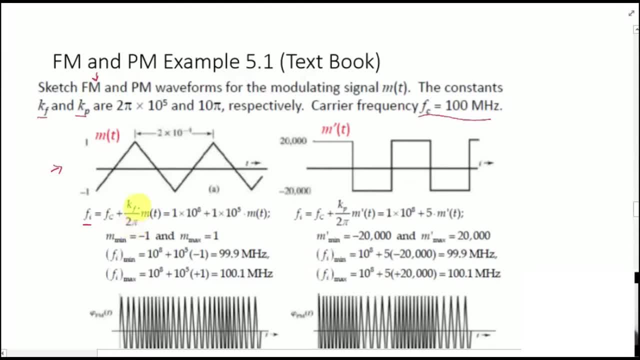 frequency rather than radians, per second omega. So Kf over 2 pi times m of t. So this K of f is given to us, which is over here, and this is the value for that 2 into 10 to the power of 5.. 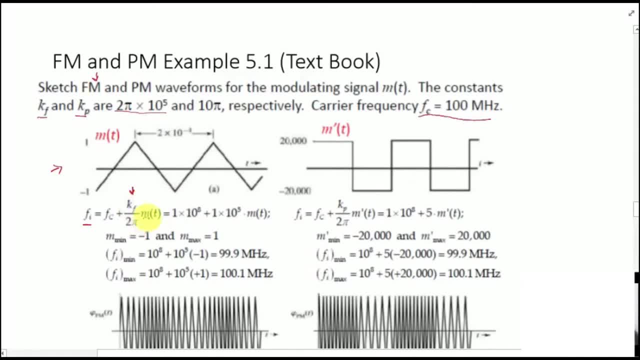 And then we divide it by 2 pi and then we see the message expression Where it lies, Just to simplify. so we have 1 to the power 8 plus 1 into 10, raised to the power 5 times the message signal. 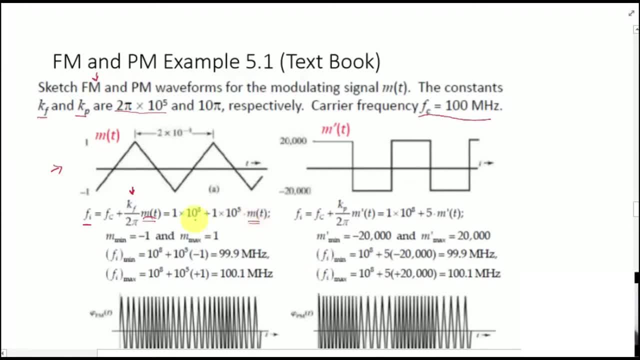 So we can see that the maximum value and the minimum value of m of t is plus 1 and minus 1.. So the instantaneous frequency, similarly, would have a minimum value and a maximum value. The minimum value will correspond to the minimum value of the message signal. So what I'm trying to say is that over here, 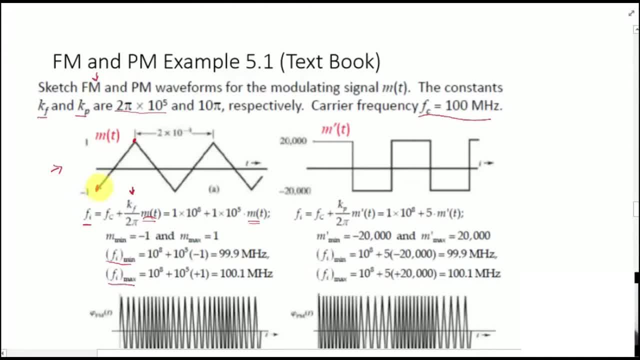 the frequency of the modulated signal would be minimum and over here the frequency of the modulated signal would be maximum. By that we can just simply plug in the values of m of t Initially. for minimum we will plug in the value of minus 1.. 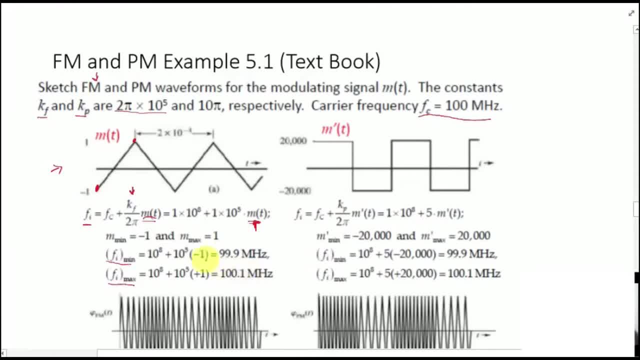 So once we plug in the value of minus 1, so we would eventually have 10 power 8 plus 10 power 5 into minus 1.. So we would have around 99.99 MHz. Remember, this is 100 MHz. 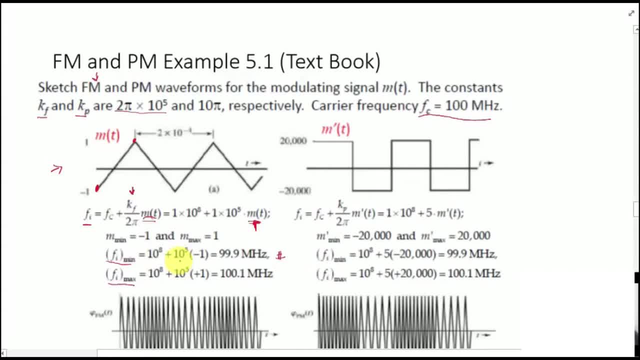 So we are removing 0.1 MHz from 100 MHz, So we get 99.9 MHz. Now for the maximum value, Fimax, we will be looking into the peak value which is over here For that. in 100 MHz we will add 10, power 5 and we'll get. 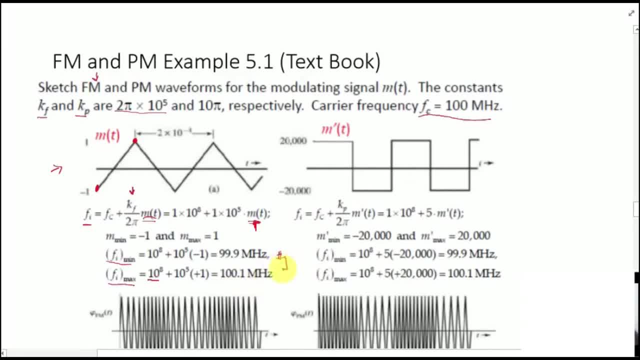 100.1 MHz. Now, remember, this is a range of value, not some crisp value. So what I'm trying to say is that over here, when we get a modulated signal that would have a frequency of 99.9 MHz, At this point it would be exactly 100 MHz. 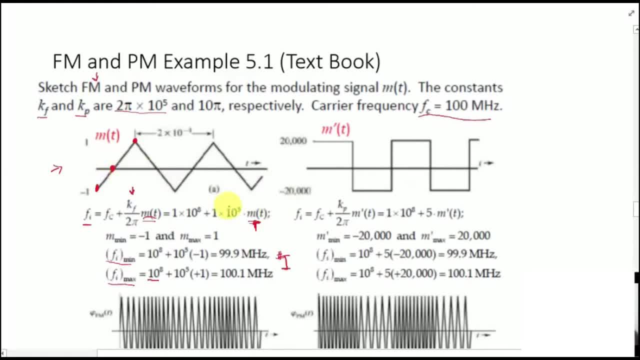 because at this point the m of t would become 0, and hence you would simply have 100 MHz, and eventually you would have over here 100.1 MHz, and then it will fall back to again 100 MHz, 99 MHz and so on. 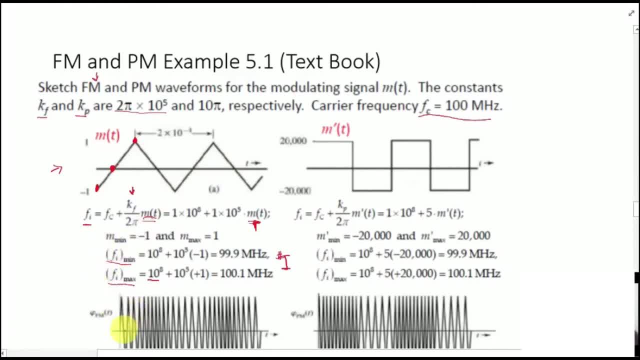 Right, so this plot is basically over here. So initially we have a low frequency and if you see, here the frequency gets quite, the oscillations quite increase until we reach m of t with the mp of t, with the peak value, and then it starts to fall down over. here You have minimum value. 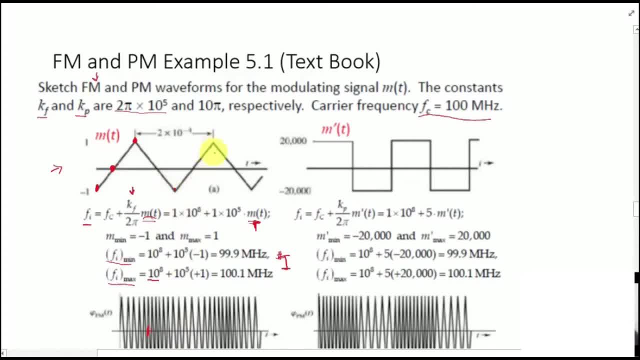 which corresponds to this value, and then again it would increase and then it would decrease. So this is basically the plot from here, which is a quite simple, straightforward plot of frequency modulation. So just you have to look into the message signal and from the message signal 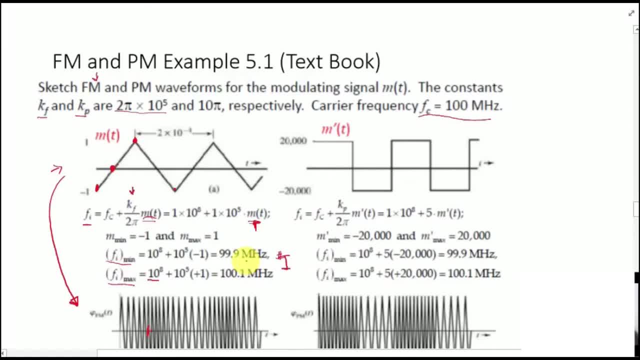 you can simply plot the frequency modulated waveform. But when we need to find the modulated waveform for a phase modulated signal? so the first thing is that we need to find the derivative of the message signal. So how do we find the derivative of it? 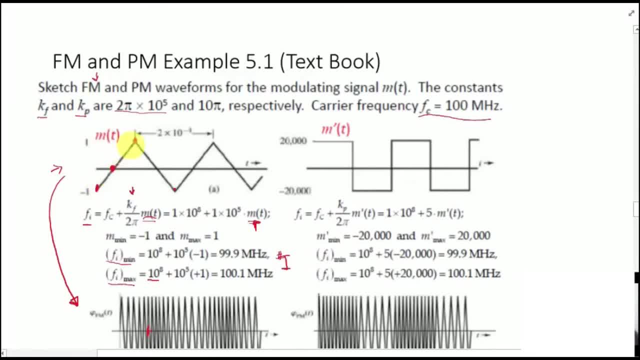 So let's. the easy way is to just find the derivative of the wave form. There's only one way is to just find the slope, And the slope is going to determine the value of the peak value of the derivative of this message. So, considering, now that you have, 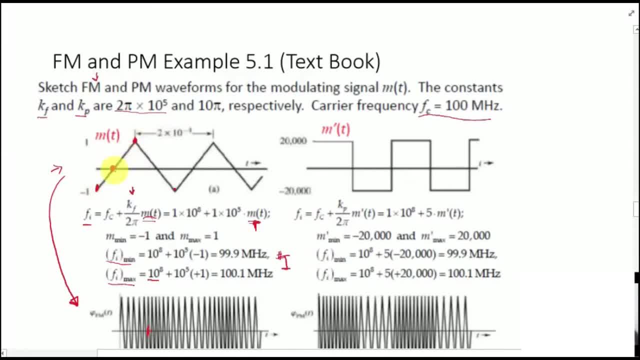 this is y2.. This is y1 over here. Similarly, over here we can say: this is x2.. This is x1.. So if you need to find the slope s Right, So this would be y2, and this would be y3.. 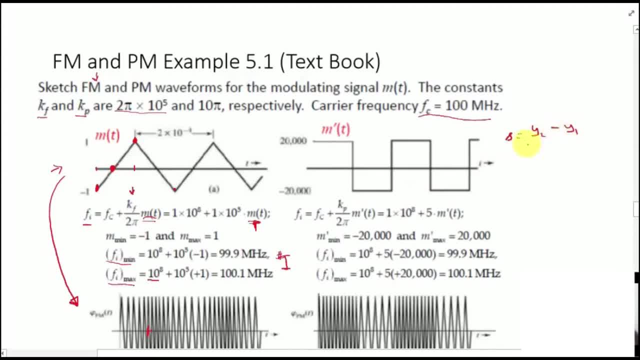 this would be y2 minus y1 over x2 minus x1.. So this is simply 1 minus minus 1 divided by So what we have is we need this value, but we know that for the bold period- that means from this point until this point- it is 2 into 10 raised to the. 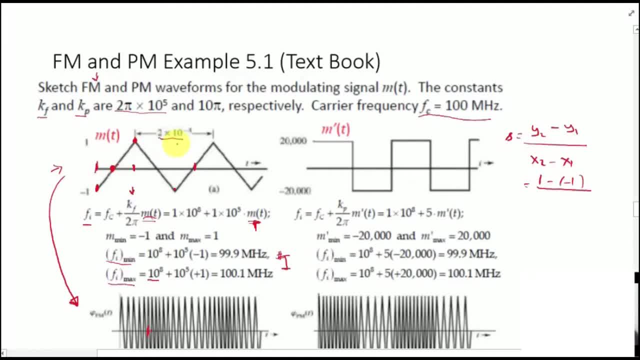 power minus 4.. 2 into 10, raised to the power minus 4.. So that is the time period. But we need half of that. So that means x2 minus x1 is half of the overall time period. This 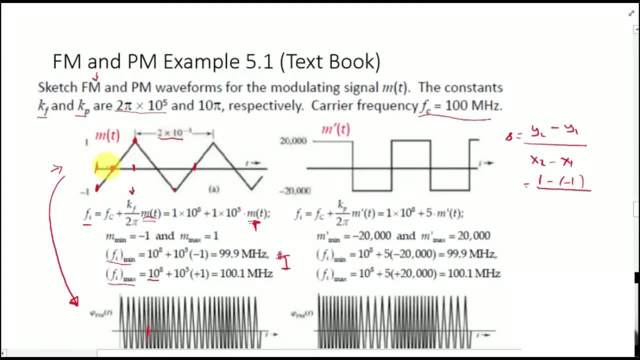 is until here. We just need half of it which lies on this plane in this range. So this would be simply 2 into 10, raised to the power minus 4 divided by 2.. So if we solve this, 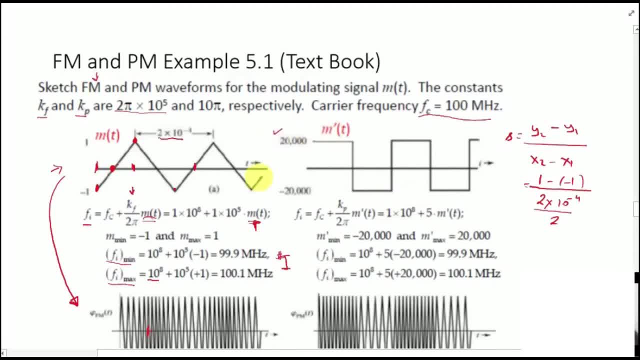 we would simply have plus 20,000 for the positive slope and similarly, for the negative slope, we would have minus 20,000.. So we get the values of plus 20,000 and minus 20,000.. So that is our m? dot of t. 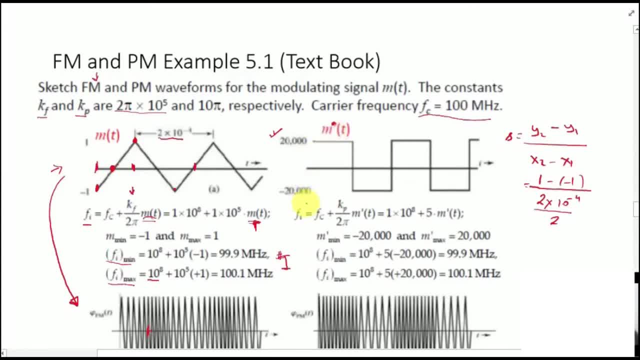 So what we are going to do is we are going to take the values of plus 20,000 and minus 20,000.. So once we got m dot of t, so the instantaneous frequency, then it is straight forward. The instantaneous frequency is equal to the carrier frequency plus kp, the sensitivity. 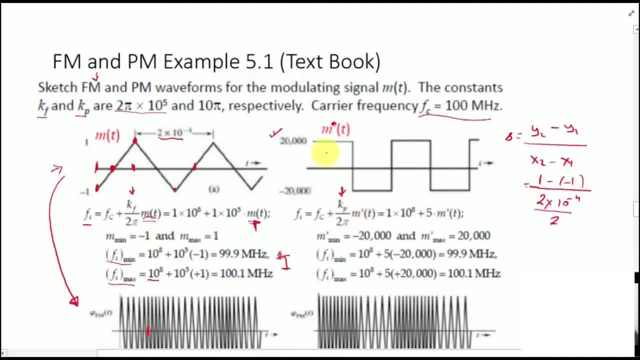 divided by 2, by m dot of t, which is over here. So the maximum value that you can see is 20,000.. The minimum value is minus 20,000.. So it is quite easy now to plot the phase. 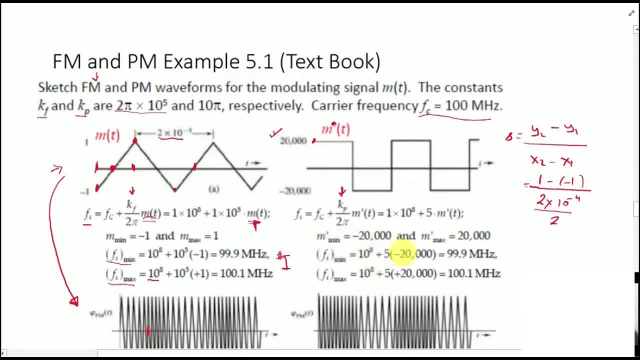 modulated signal. You would just plug in the negative value, So you get the minimum frequency, which is 99.9 megahertz, and then you can plug in the positive 20,000.. So it is going to give you. 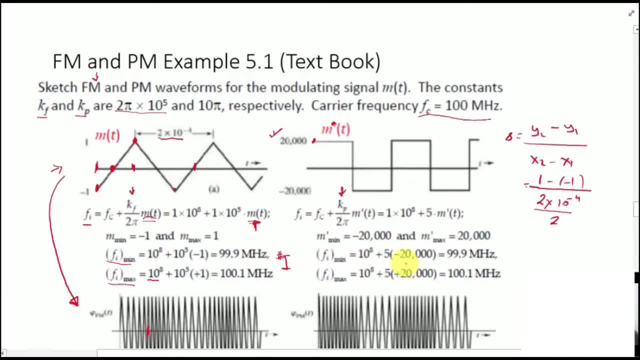 100.1 megahertz. So an important point over here is that for this signal you simply have consistent frequency. Over here you would have a low frequency. Over here you have a high frequency and low frequency, Whereas for frequency modulated signal it was basically. 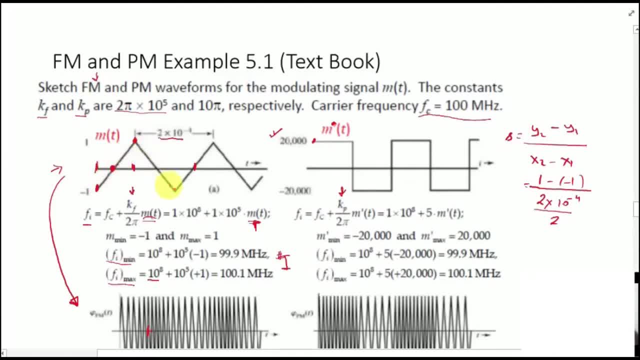 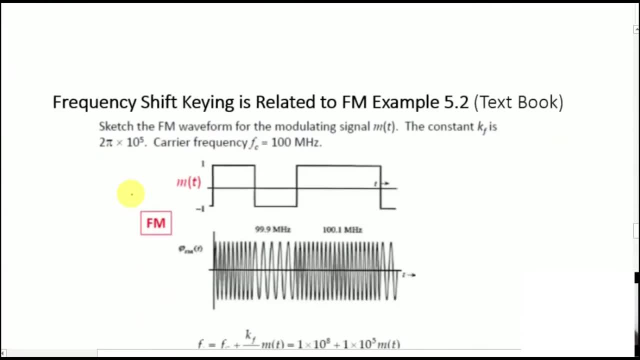 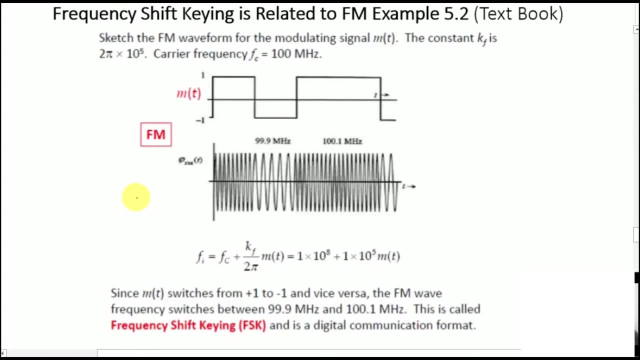 decreasing linearly and then decreasing and so on and so forth. So this brings us to another very, very fundamental aspect of communication, but this time it is more related towards digital communication, where we use the word shift keying. So you could say shift keying is used in parallel in digital communication. For example, if 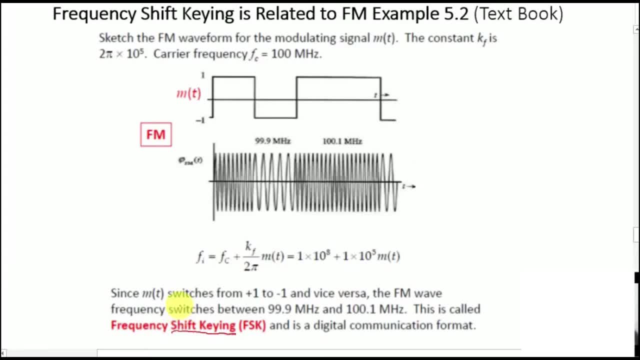 as compared with analog communication, where we use modulation. so in analog we often use modulation, whereas in digital communication we are more, uh, we are specifically concerned about shift key. so presently what we have is: uh, this is example 5.2 in our textbook, so it says that we need to. 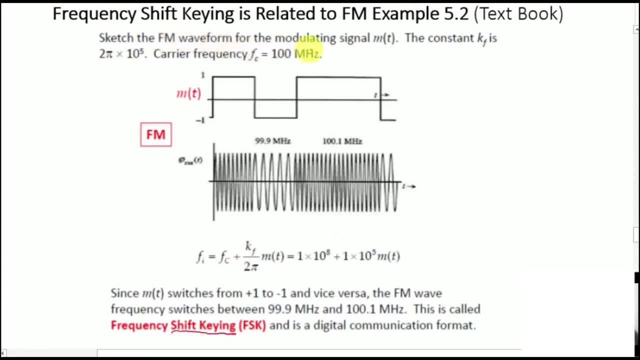 sketch fm requesting modulated waveform for the modulating signal m of t, and then it is giving us a constant kf which is two, two pi times four pi, and then again the carrier frequency is 100 megahertz. so it's quite obvious that now the method signal whenever it is plus one. 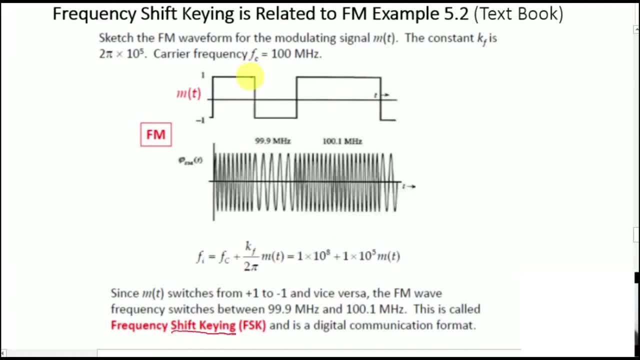 you would have m value, m peak value of plus one or m max value of plus one, and then you can have a min value of minus one whenever it's plus one. uh with hundred would be added with kf times plus one, so you would simply have uh, this uh on this expression. so if you put plus one here, 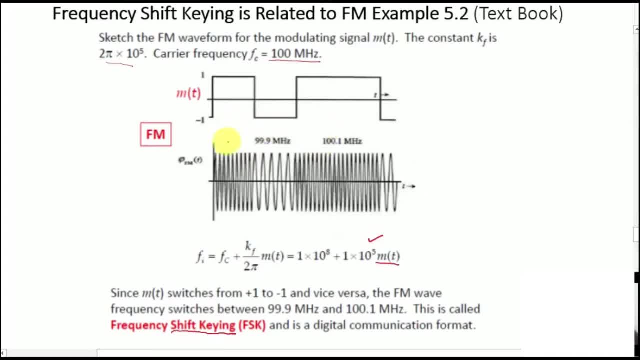 you would have a hundred point one megahertz over here, and then you, if you put uh m of t equal to minus one, you would have 99.9 megahertz. so, depending on the input signal, you, uh, you're going to shift, key it into a specific frequency. now, when we are specifically mentioning digital, 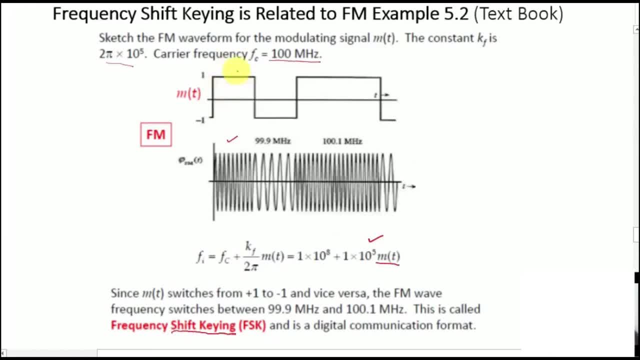 communication, the format for our signal might be in terms of ones and zeros, so we may have something like a one here, a zero here, which is represented by a minus one volt, or again a one and a one. so plus one volt is represented by 100.1 megahertz and then a zero is represented. 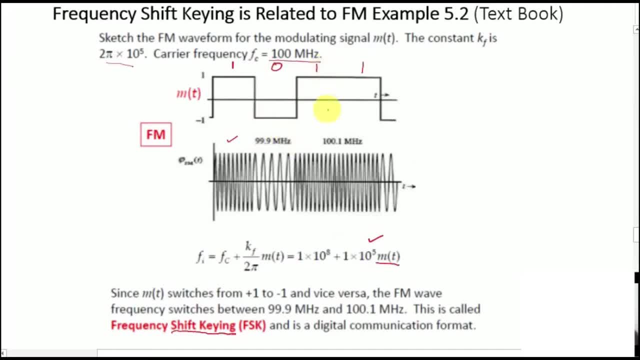 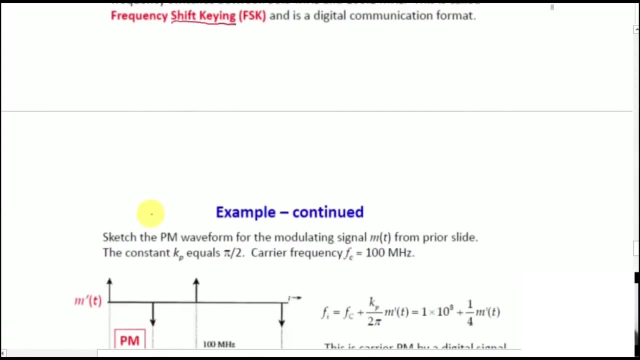 by 99.9 megahertz, and again plus one is represented by 100.1 megahertz. so this type of translation is something that we call that fsk, which is frequency shift in, uh, digital communication systems. now, next it says that we need to sketch a pm. now this really gets. 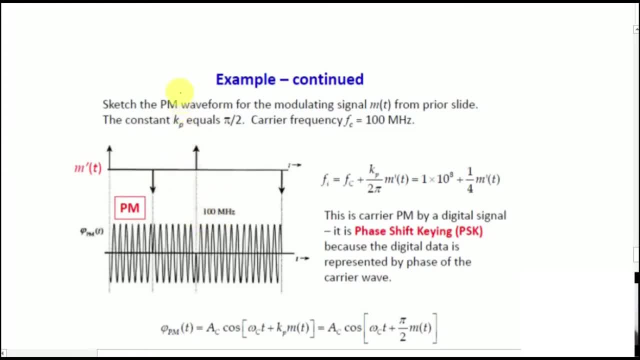 very, very interesting. so it says that we need to sketch pm phase modulation waveform for modulating single moft. so, considering it, it again gives us, uh, some constant value, kp, which is equal to pi by two, and the carrier frequency is the same, which is 100 MHz. Now for the given message signal. if this is the M of T. 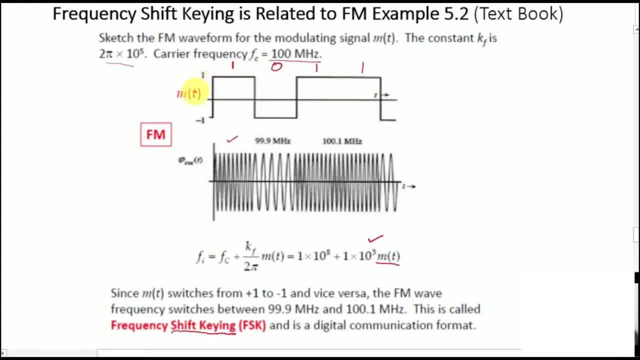 the first thing is, of course, for PM we need to take the derivative of this one. So if you take the derivative of this one, you can see that there is an increase from minus 1 to 1.. So you would have an impulse here which would have a strength of. 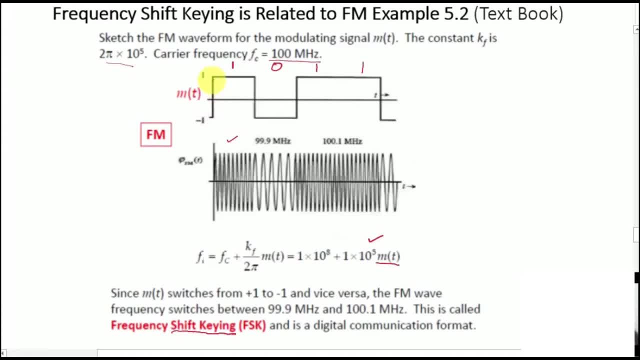 2, right plus 2. But over here the slope remains 0. So there is no change. So over here the value would be 0, and then there is the negative slope of strength minus 2.. So in a way, when you take 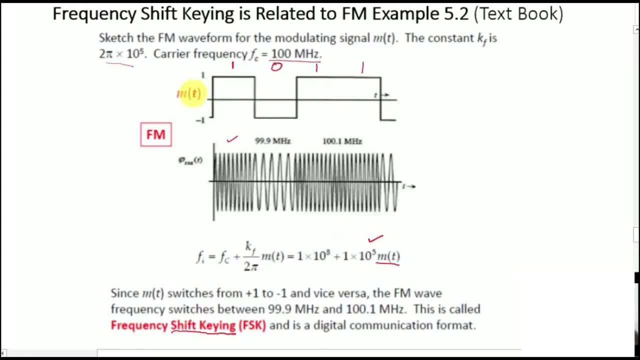 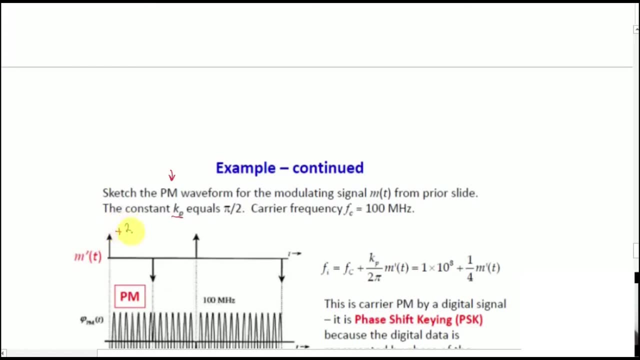 the derivative of this message signal. so what you would have is you would have a plus 2, a minus 2 here, again a plus 2 here and a minus 2.. So this is basically plotted over here. So M dot of T is a delta function of having strength plus 2, and then a delta function of 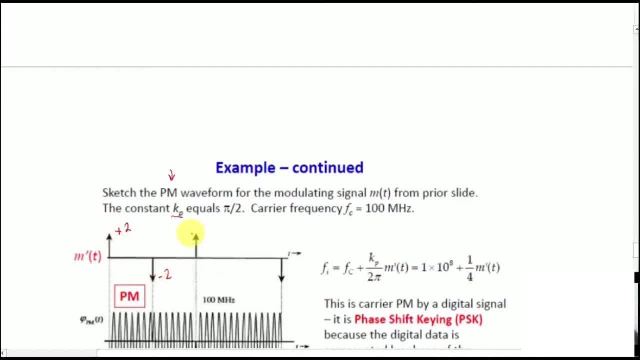 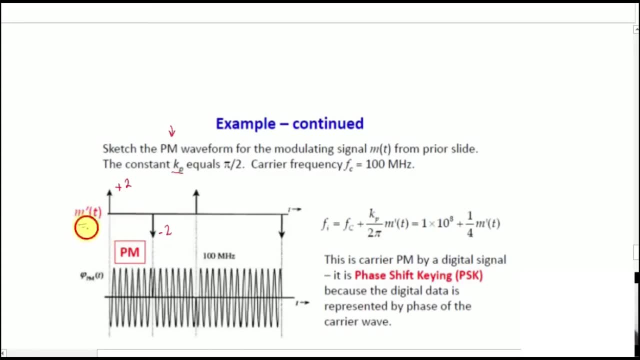 having a strength of minus 2, and so on and so forth. right, So once we get M dot of T now, we can calculate the instantaneous frequency fi of T, which is f c plus k p, the constant divided by 2 pi, into M dot of T, which is again this: 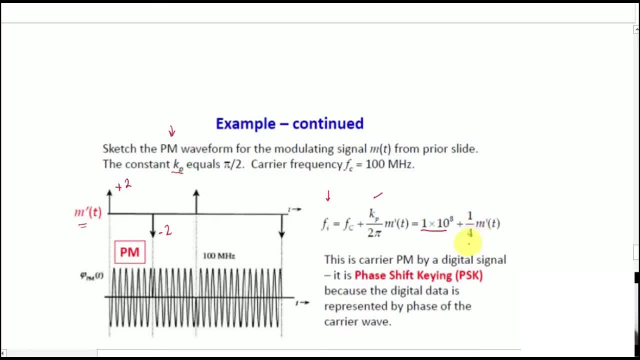 is 100 megahertz and this is simply 1 by 4 m dot of t. it's basically the frequency is not changing right now, it's simply 100 megahertz. so but what we have difference where we differ is that wherever we get a spike or a delta function, we would have a phase change, and presently that phase change is 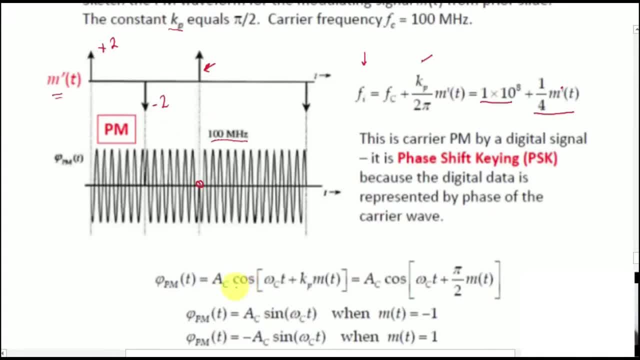 of 180 degree. i will elaborate further. initially, when we are sending a signal, we have something like: p? m is amplitude of the carrier, cos times omega c, t cos, with argument: omega c t plus k p, m of t, right. so this k? p is something that what you call that. 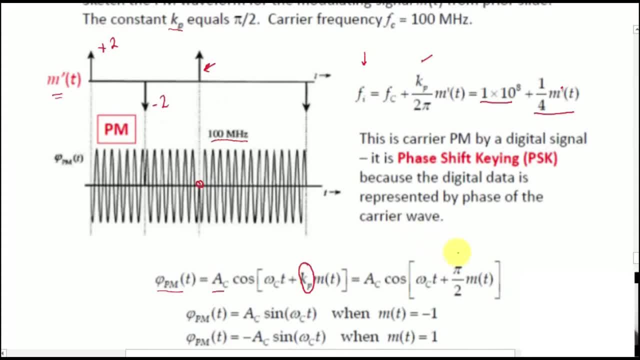 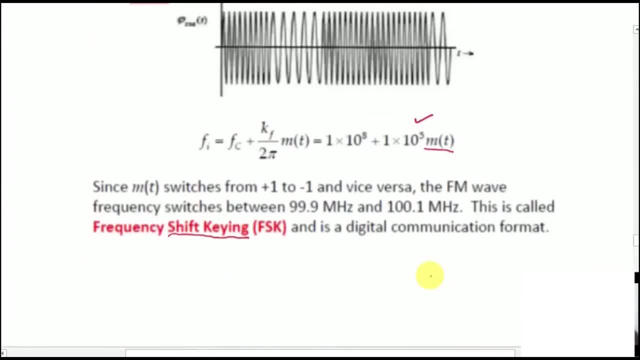 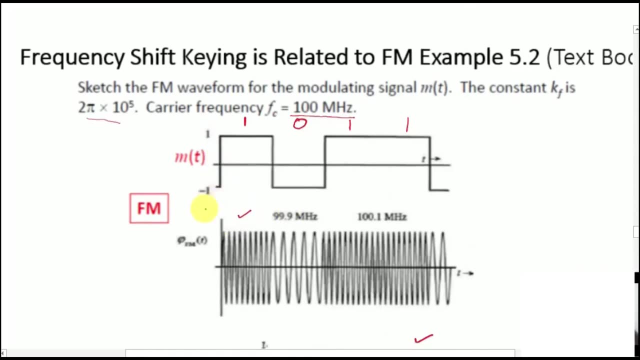 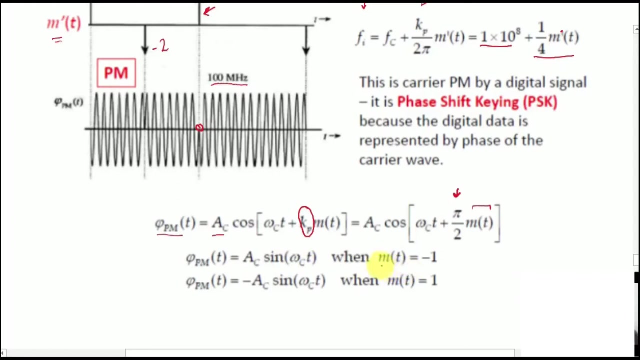 is the sensitivity constant. so now this is given, which is pi by 2, and then we have a message signal m of t. remember originally that the message signal was either plus one or it was simply minus one. so it was plus one or minus one. so the message signal would be either over here i have mentioned minus one or plus one. 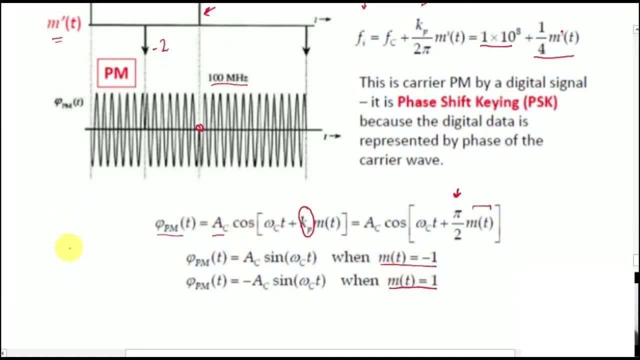 so if we want to plot this cos function, so it is, it is something like minus one or minus one. so if there is m of t which is minus one, so that means omega c, t minus pi by two, so by minus uh, by a phase shift of minus pi by two. what we mean is we mean that 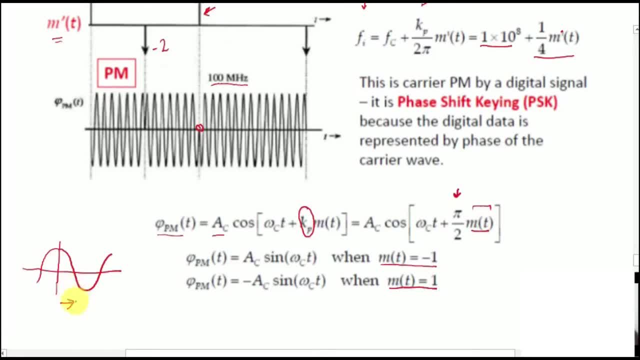 we are going to shift this signal towards right. right. so minus pi by two would mean that we will are having something like this: So this would convert to ac, sin, omega, ct. But when we are having m of t equal to plus 1, so if you plug in the value of m of t equal to, 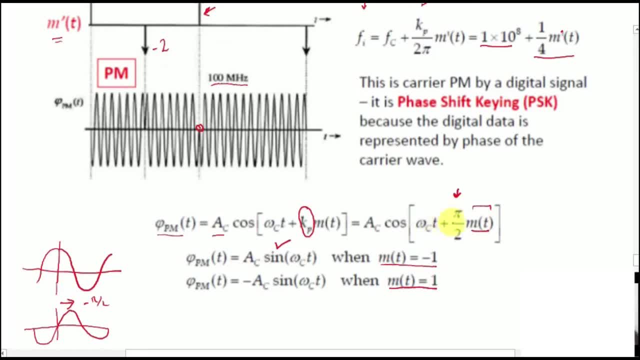 plus 1, so this would become omega ct plus pi by 2.. If you have plus pi by 2, then the waveform would be shifting towards left and hence you would have: so this is simply minus ac, sin, omega ct. There's a phase shift of pi, which is: 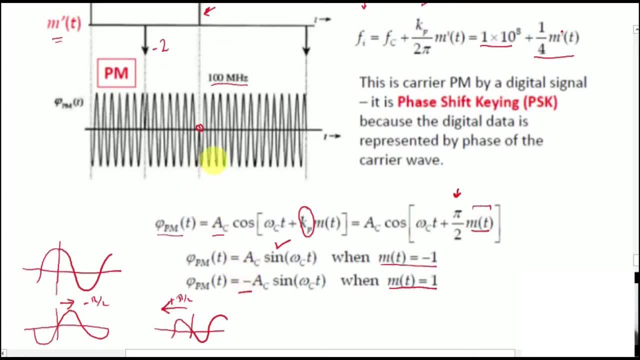 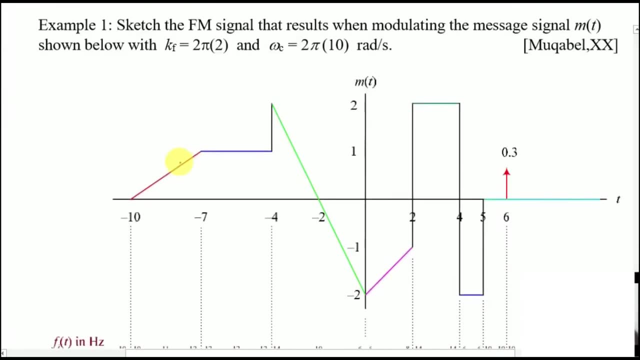 plus ac, minus AC, sin omega Ct, which is basically observed over here. So this is phase shift key. there is a phase shift of phi whenever there is an impulse. Now the next example is actually even more interesting, So there are two more examples. 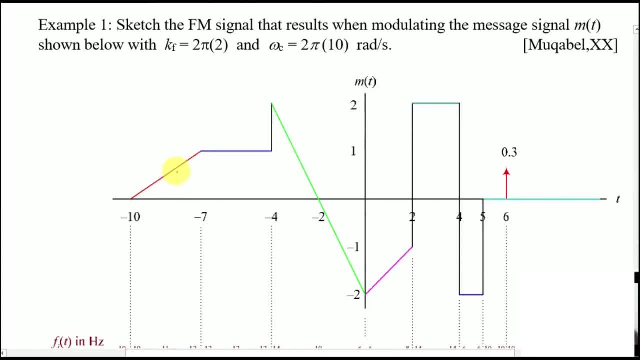 that we'll do next. So in the first example we are given this signal. this is our m of t and it is rather involved. We can observe that the message signal m of t. it starts at time minus 10 and then it continues on until 7, where it remains the same, and then there's a. 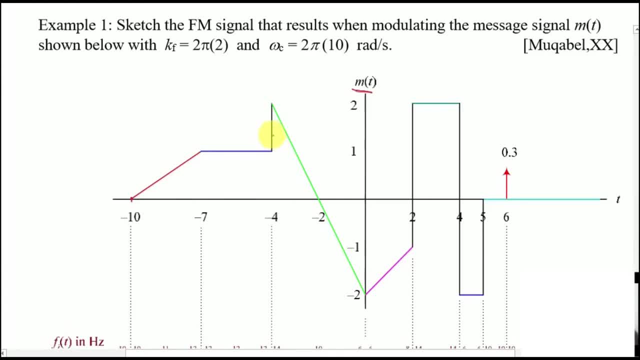 jump discontinuity at minus 4 and then there's a gradual decrease and so on. And, importantly, we have a delta function. So whenever there's a delta function, things get really interesting. Remember that we are asked to sketch an FM signal and for that we are given. 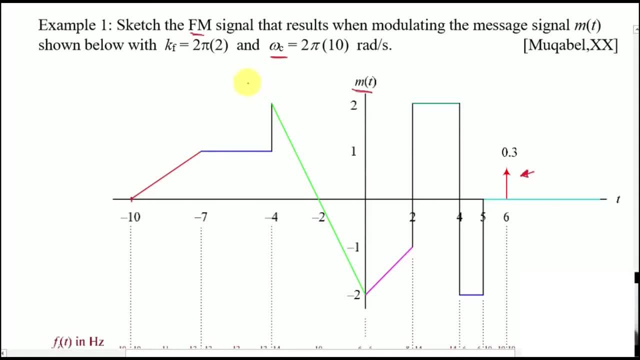 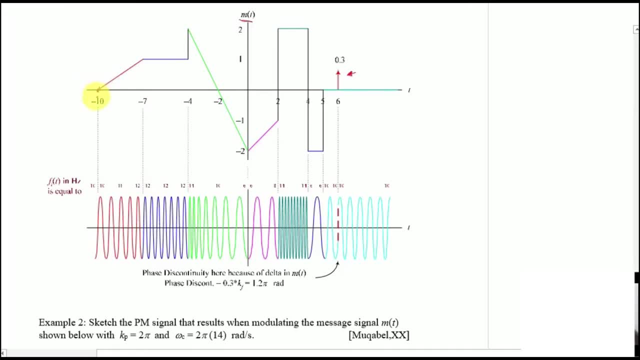 angular frequency. omega C carry frequency and sensitivity: constant Km. From this point. at this point, the value would be the value of oscillation. the oscillating frequency would be exactly equal to omega C, But as the value of message signal increase, so would the instantaneous frequency. So overall, the oscillation would 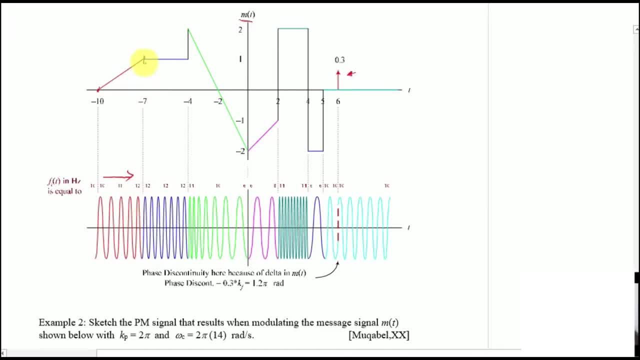 decrease until this point. So once we reach here, from this point to this point, it would remain the same. So once we reach here, from this point to this point, it would remain the same. The instantaneous frequency would remain the same. Then there's a discontinuity over here. 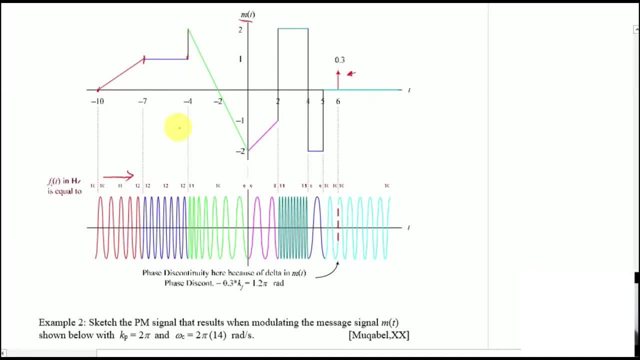 and then from here suddenly the frequency would increase at this point over here, but then it would gradually drop. The instantaneous frequency would become low Over here. it would increase, and then it would suddenly jump up and increase further. Then it would drop down. 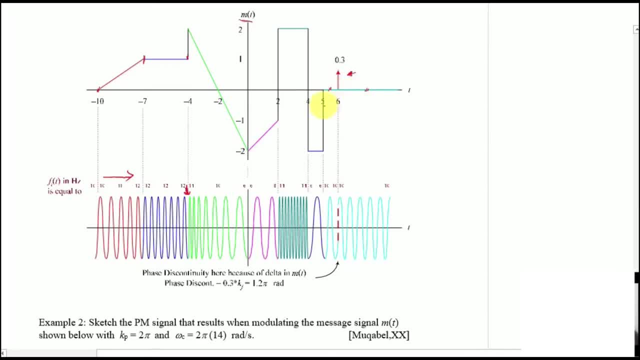 Over here this would on this range, we would have simply omega C, and over here we have a direct delta function, direct delta function. So let's interpret it further, further. So some of the things are quite obvious, Whenever, 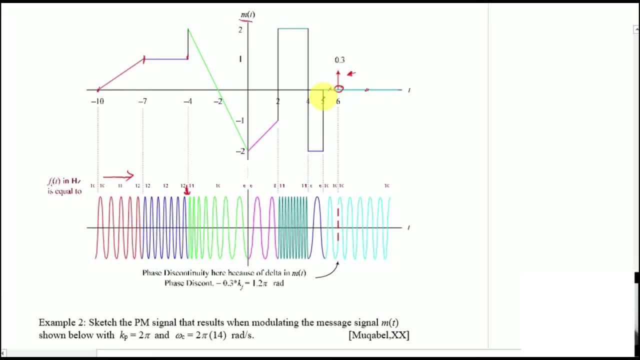 the magnitude of the message signal is high, the frequency would be higher, And whenever it is low, it should be lower. But the interesting things are when we have, when we are faced with a delta function. so we have a delta function here which is having the strength of 0.3. so remember a delta function. 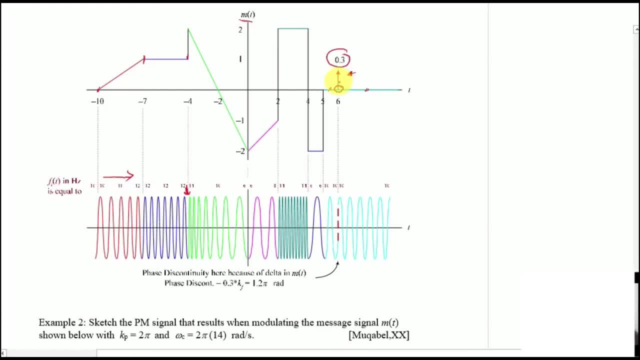 has approaching zero width and infinite height. so by 0.3 we mean that its area is equal to 0.3 right. so over here, when we have discontinuity, we would have a phase shift Right and its called phase discontinuity. so this phase discontinuity is nothing but. 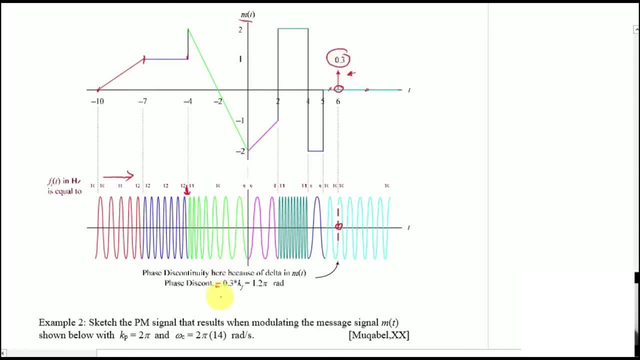 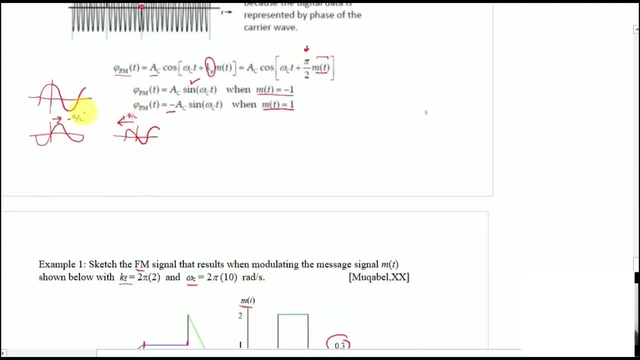 the strength of this direct delta function, which is 0.3 Times kf. so this is equal to 1.2 Phi RadiusSo, as discussed before, The amount of shift that you would get. so this is what we would have. this is the the aspect�� 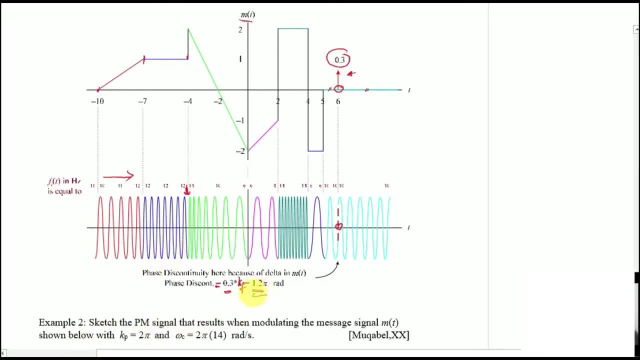 amount of shift that we will get, which is 1.2 pi, and this is observed over here by means of dotted lines. okay, so the another important consideration is when we are here, or, more importantly, when we are here, you can observe that this blue- uh, the blue signal and the green signal. 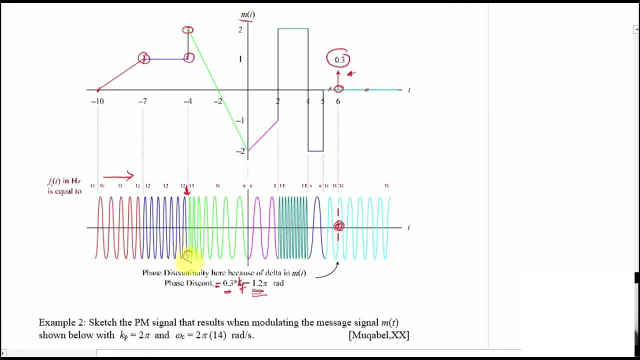 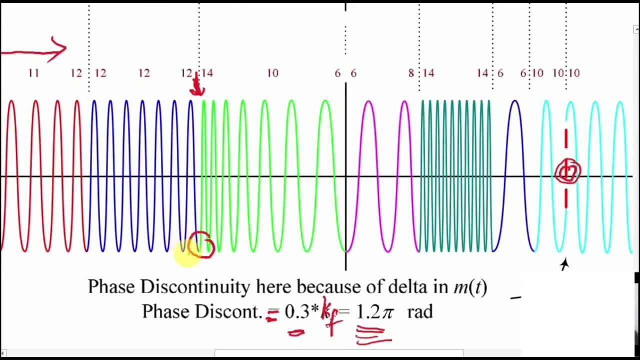 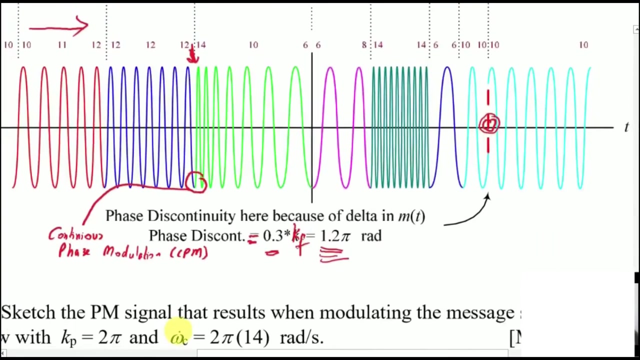 they are combining at this point, so let me zoom it further. if you see, there is no discontinuity over here, the blue will finish here, blue waveform will finish here and then green will stop. this is something that we usually term in communication as continuous phase modulation, cpm. continuous phase modulation- right, and it plays a very, very significant role. 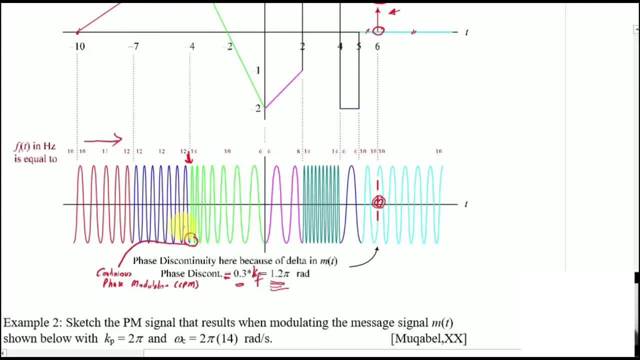 because if you have discontinuities in a signal, so what it would do is it would create a a big number of harmonics and you would have quite high frequency and we need to avoid it. so we need to avoid this kind of scenario, but anyway it. 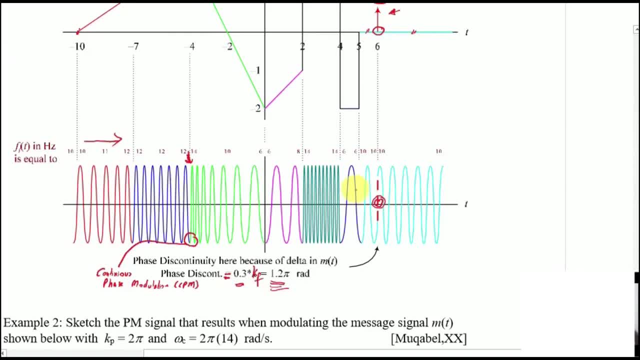 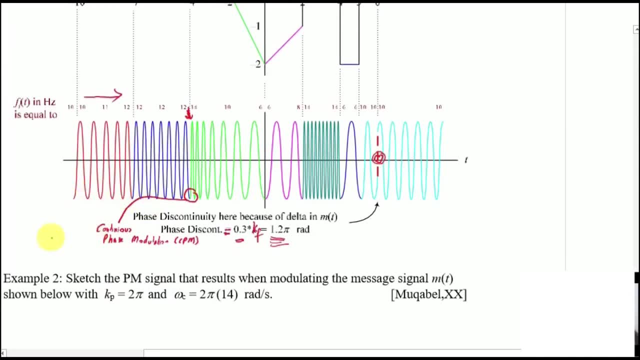 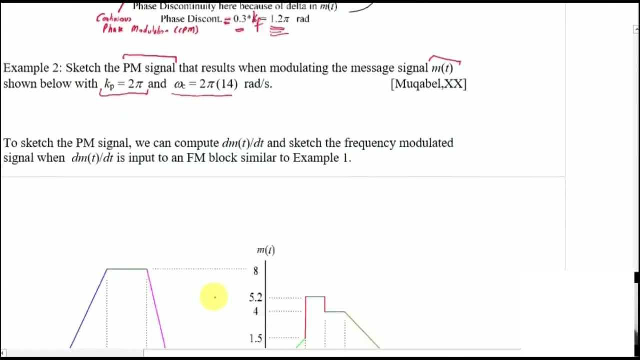 if we are faced with a signal in which we cannot avoid it, so we can't help it. next, this is a desire to sketch a pm signal. and then we are given a new message signal m of t, and we are also given a given the constant kp, as well as angular frequency, omega c. 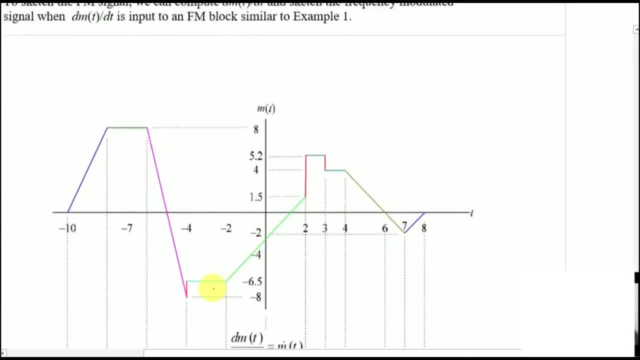 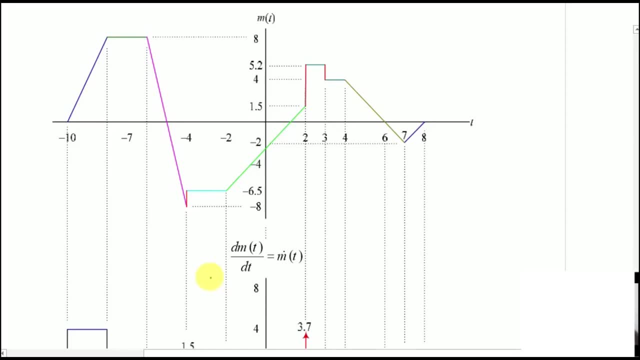 So we are asked to plot the phase-modulated signal. Again, we have the message signal. first thing that we would do is take the derivative of the message signal. So whenever there is an increase in the magnitude, we would have a value of slope which is represented. 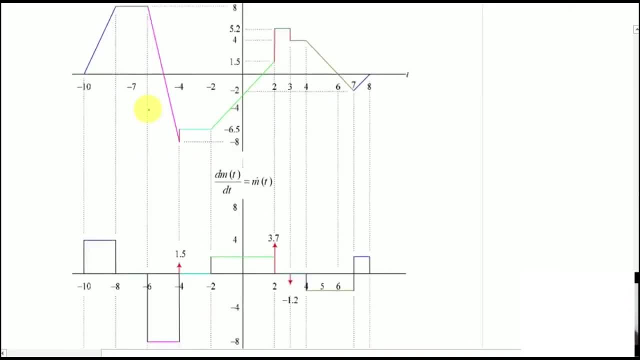 here. So, similarly, over here the slope would be 0, so our value would be over here 0. And then it is decreasing, so our value would be decreasing, but then there is a discontinuity here. So, once we are taking a derivative, so this would be basically showing direct delta function. 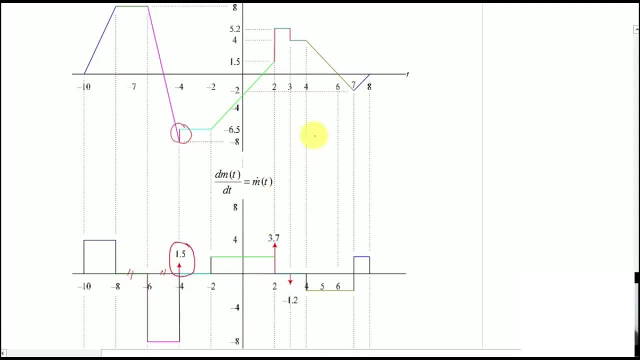 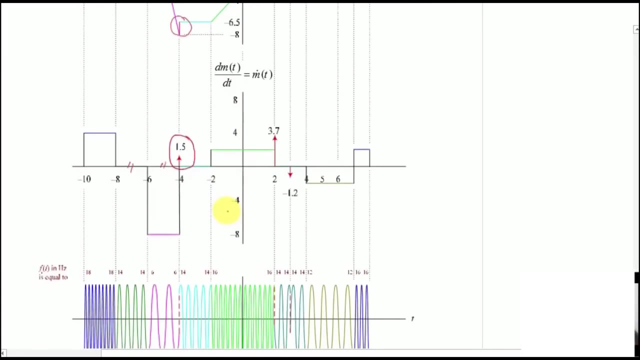 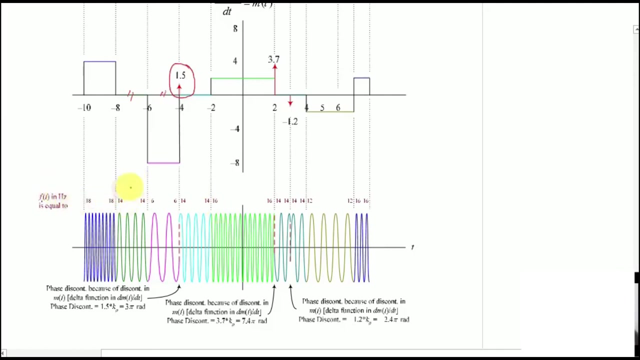 of strength 1.5.. Similarly, we are also having some discontinuity over here, Okay, Right, And here and so on. So next, when we are going to modulate it as per the prior discussion, So over here, the pattern before this one, you would simply have omega c. 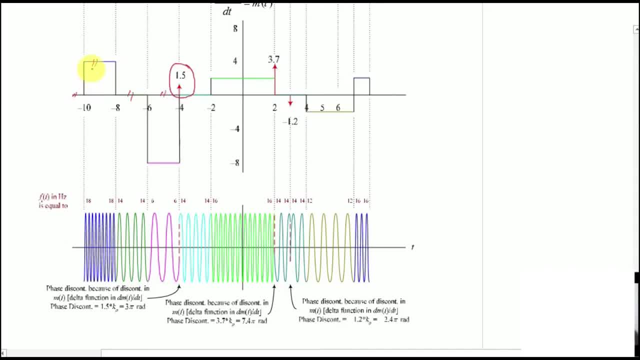 Over here you would have omega c plus kp by 2 pi into omega c. Again over here you would have omega c. Here you would have omega c plus kp into minus 8 and so on. But over here we would have a discontinuity. 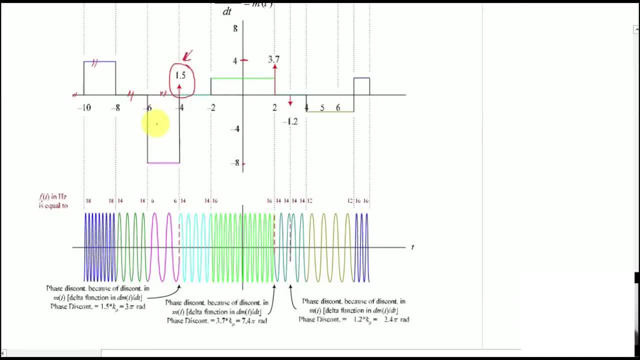 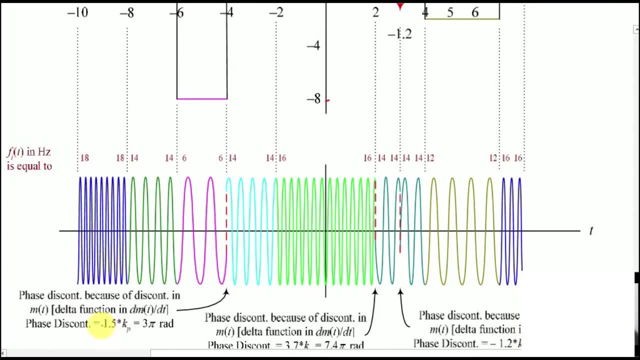 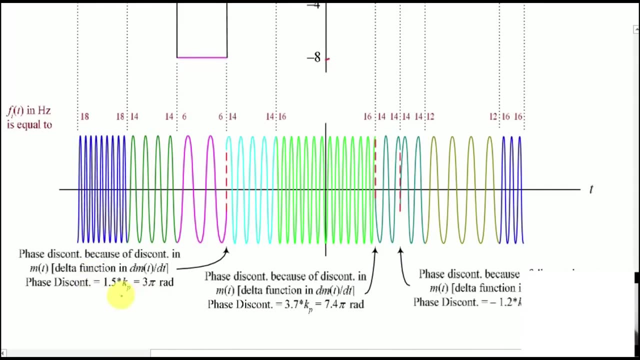 So this is simply 1.5, which is coming from the strength of it. And over here, you would have omega c plus kp by 2 pi into 2 pi. So we have an 최 � ovat consequence. length of it 1.5 times the sensitivity constant which is kT, this is 3π radians. 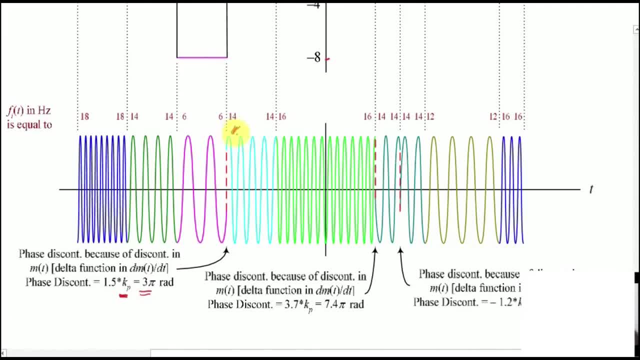 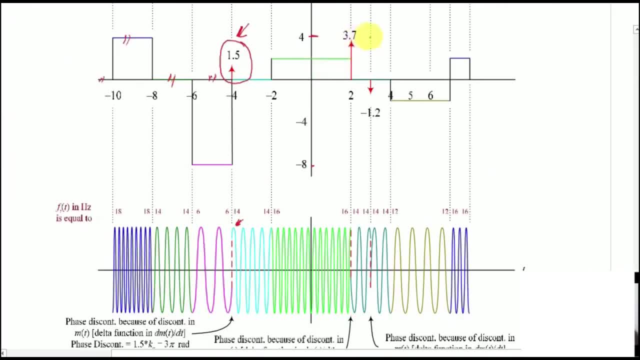 So the phase shift would be of 3π right And similarly, whenever we have a direct delta function, we would have a phase shift, and this is represented in all the blocks right. So eventually we would have this signal, which is: 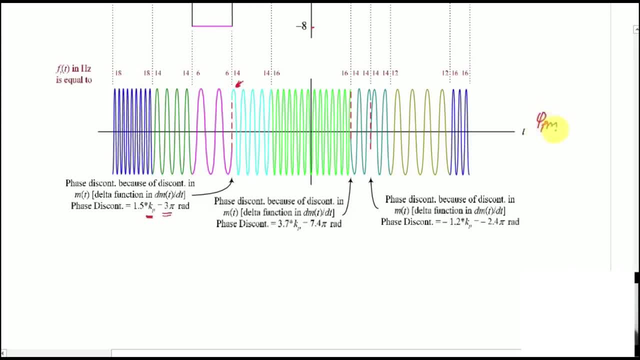 basically phase modulated signal in time domain.